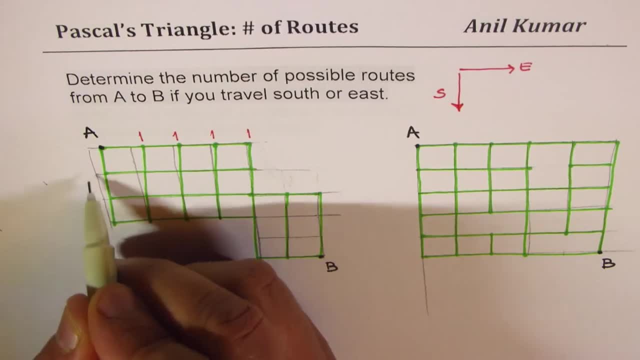 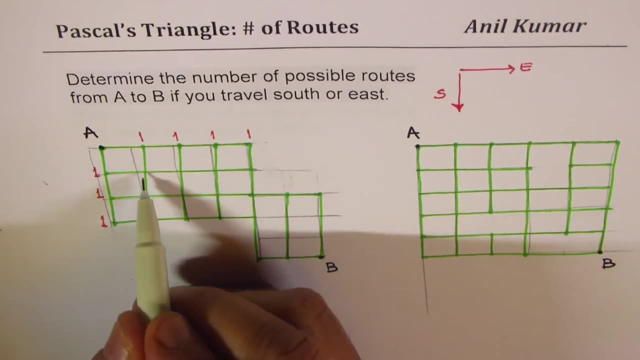 the south side. there's only one way going south, so I can write this as 1,, 1 and 1.. Now, if I have to reach this point, I can reach from two places, correct? Since I can reach from these two, we'll add those numbers, and so we get our number 2 here. So I hope this is. 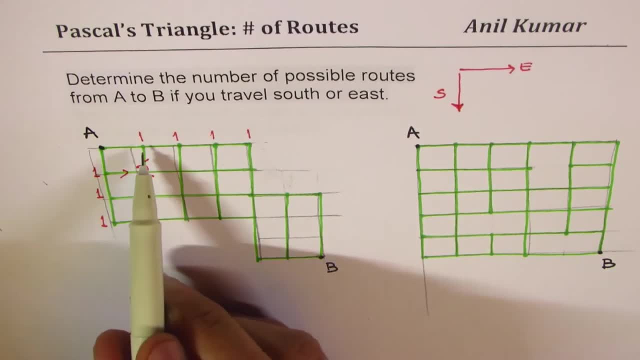 very clear how we get this number. There are two ways of reaching this point. One is east and then south, and the other way is south and east. These two ways are represented by number 2.. How about this position? Now, there are two ways to reach here, So we have third, So it is 2 plus 1.. 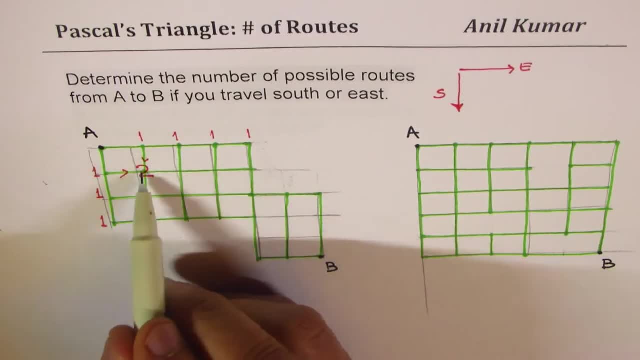 You could reach from this side or from there. So add these two numbers to get the next number, which is 3 for us At this place, 3 plus 1, 4, and continue the process. we get 5 there. Do you see? 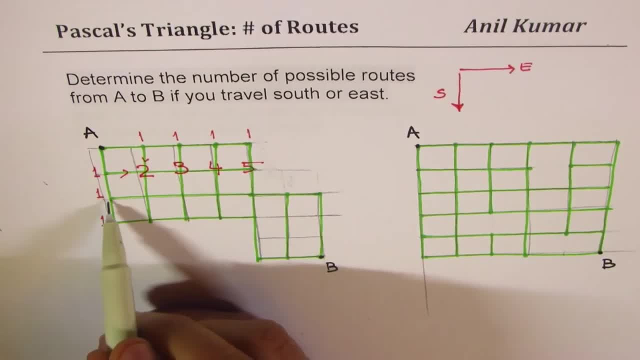 that, So it's not that difficult. Now, here we'll add these two points: You can travel only south and east, So you can come from these two places. You cannot come from there. So there should be 3 and this position: 3 plus 3 is 6,, 6 plus 4 is 10,, 10 plus 5 is 15.. You can go straight. So those 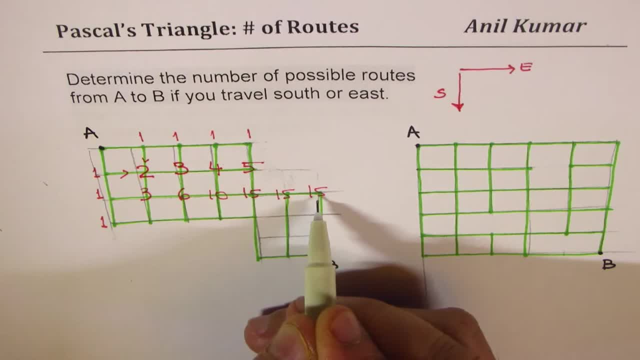 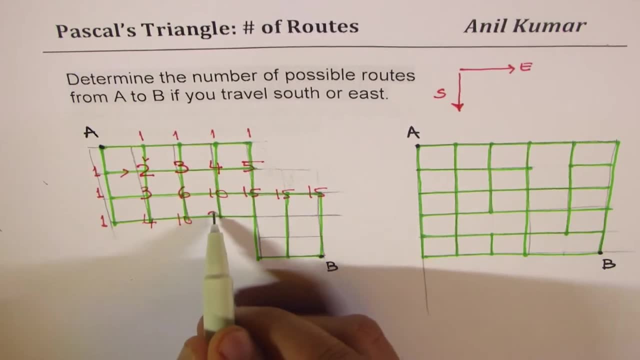 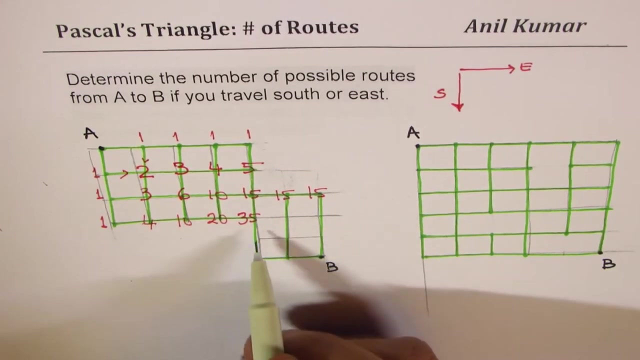 will also be 15.. This is critical to understand. Is it okay In this place? 1 plus 3 is 4, 4 plus 6 is 10, 10 plus 10 is 20,. 20 plus 15 is 35. So 35. If you're. 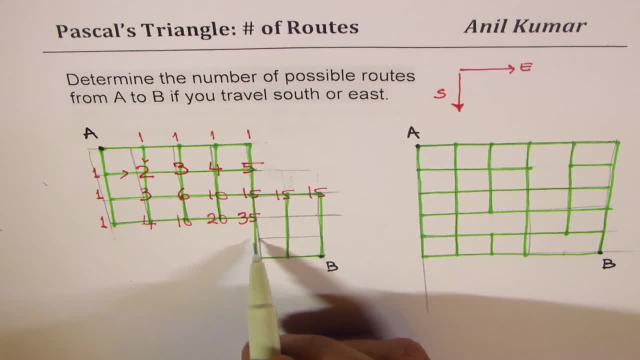 going down, those points will be 35,. right, This also 35.. Now if I'm going east, I can reach here from two positions. So we'll add 15 and 35,, 15, 5 plus 5, 10. Then we have 5 plus 5, 5 plus 5,. 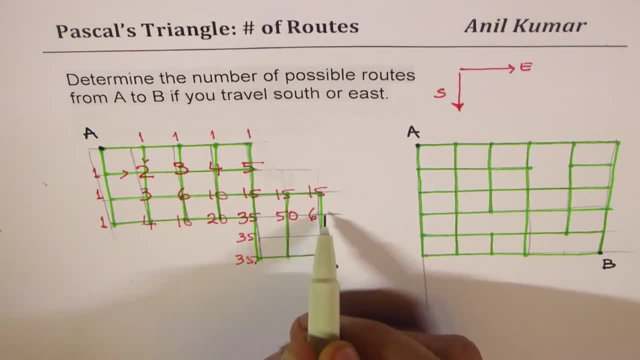 50 here. 50 plus 15 gives us 65 for the next location. Then we'll get to this: 50 plus 35 is 85,, correct, 85 plus 65, 5 and 5 is 10, and 7 and 8 is 15, 150.. Now 35 and 85, you can use. 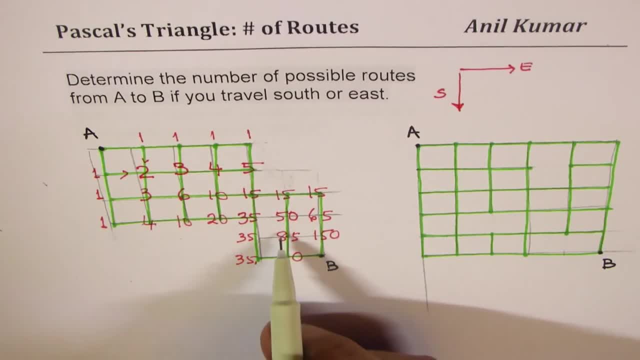 calculator 5 and 5 is 10, 1, 9 and 3, 120.. Now 120 plus 150 gives us 270.. So in all we have 270 ways from A to B. Is that clear? Is that clear, Right? So take a moment, understand this process. 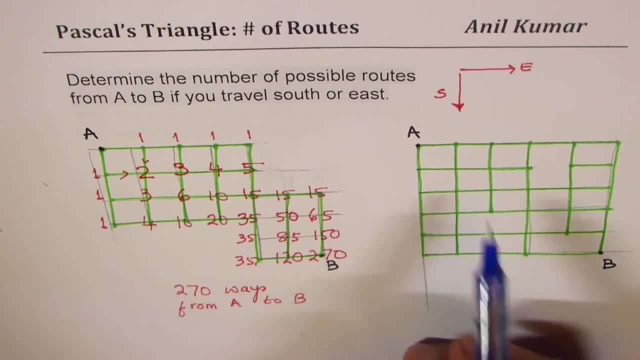 Perfect, And then do this yourself. So now there are a few blank places here, Okay, So take care of that and see how it gets modified. So, to begin with, if I'm moving east- 1, 1, 1, 1, 1. No problem. South- 1, 1, 1, 1, 1.. These points. 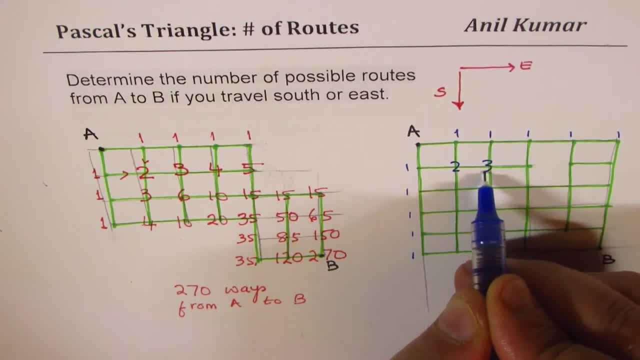 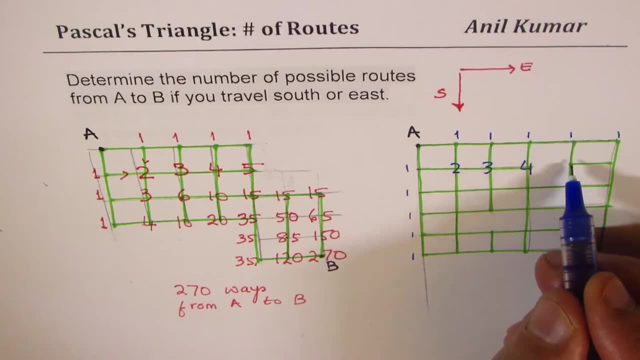 intersection: 1 plus 1, 2,, 2 plus 1,, 3,, 4, right, But here you cannot go from this side. The only way is coming down from 1.. So it is again 1.. Do you see that? And 1 plus 1 gives you 2.. 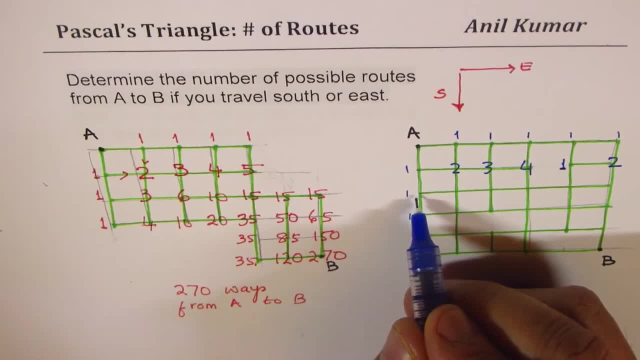 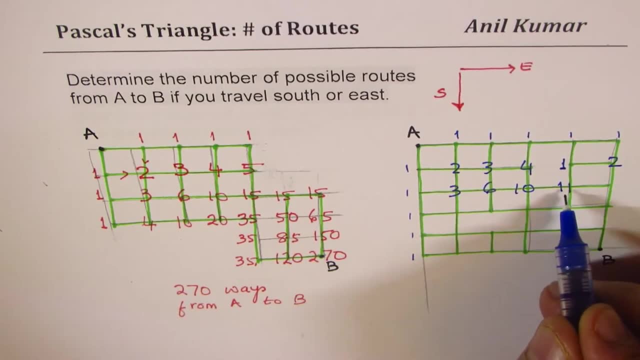 Now back to second row. 1 plus 2 is 3,, 3 plus 3 is 6,, 6 plus 4 is 10,, 10 plus 1, 11, and 11 plus 2 is 13.. 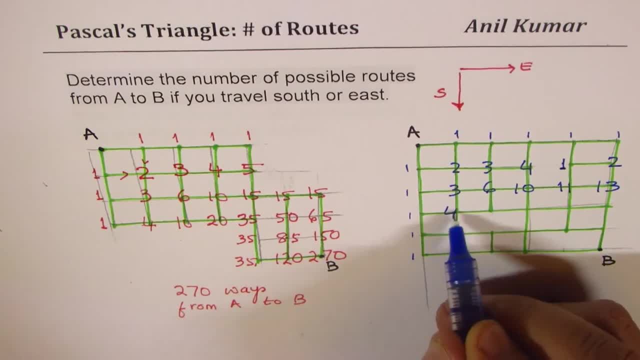 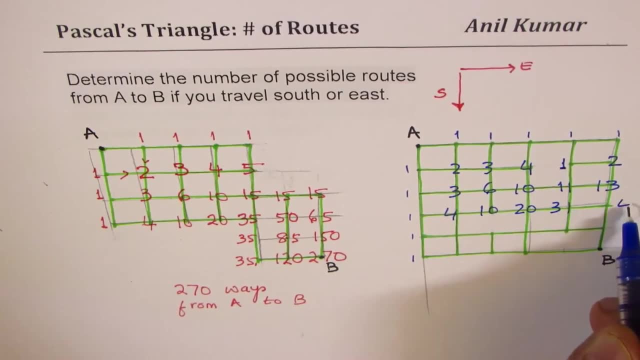 Now let's get back to this: 1 plus 3 is 4,, 4 plus 6 is 10, 10 plus 10 is 20,, 20 plus 11,, 31,, 31 plus 13,, 44.. 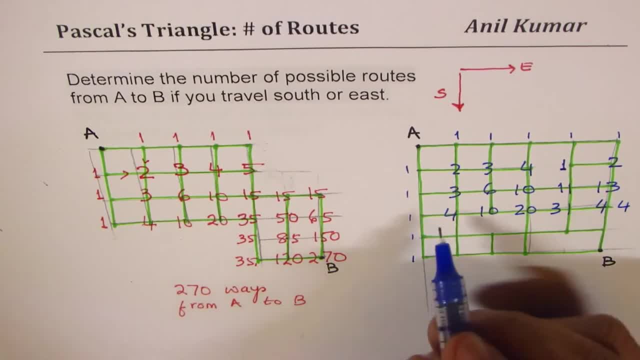 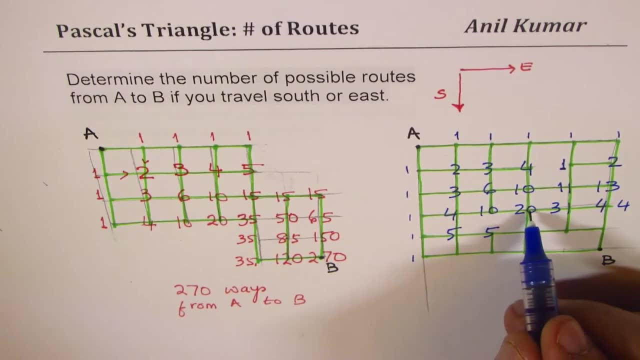 Correct Now 1 plus 4 is 5.. You cannot come from there, So still 5.. You can come from 20 now. 20 plus 5 is 25.. 31 plus 5, 6 and 56.. 44 plus 56 is 100.. Okay, This side, 5 plus 1 is 6, 6 plus 5 is 11, 11 plus. 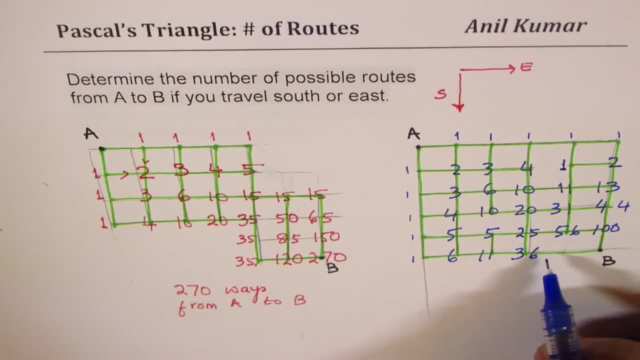 25, 36.. 36 and that's it. 36 plus 100 is 136.. So in this case we have 136 ways from A to B. Okay, So I hope the process is clear. So that was kind of a warm-up exercise, And now we have a word problem for you. 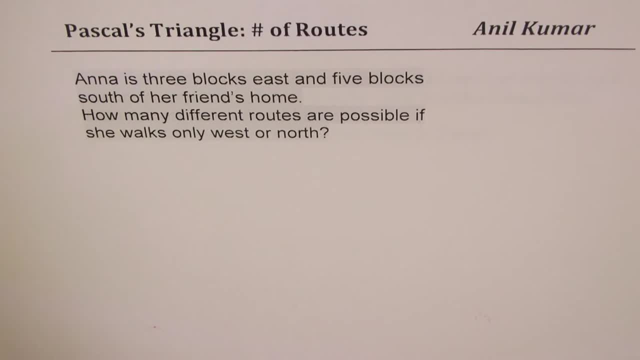 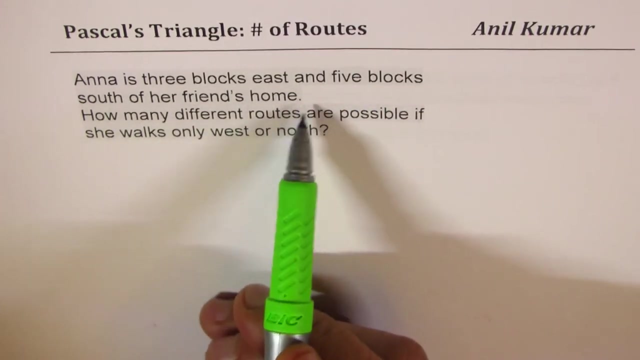 It says Anna is three blocks east and five blocks south of her friend's home, Right? So Anna is three blocks east and five blocks south from our Friend's home. How many different routes are possible if she walks only west or north? So in this case she can walk either west or 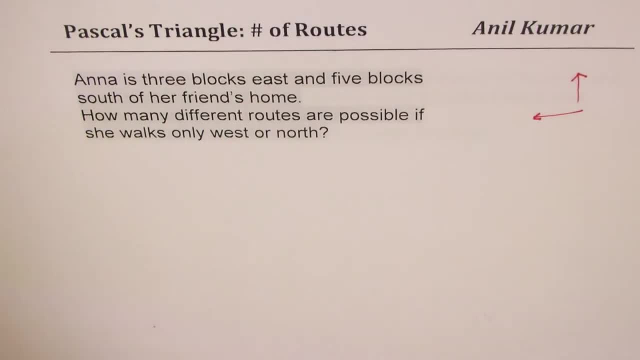 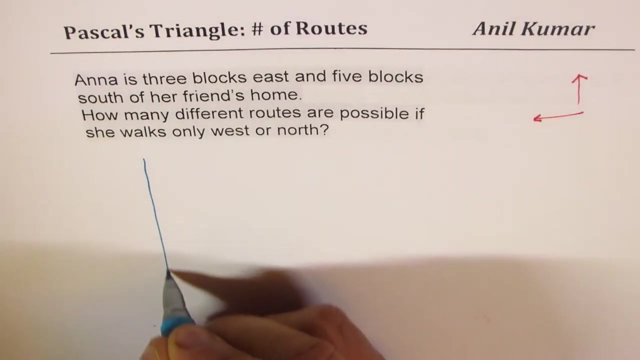 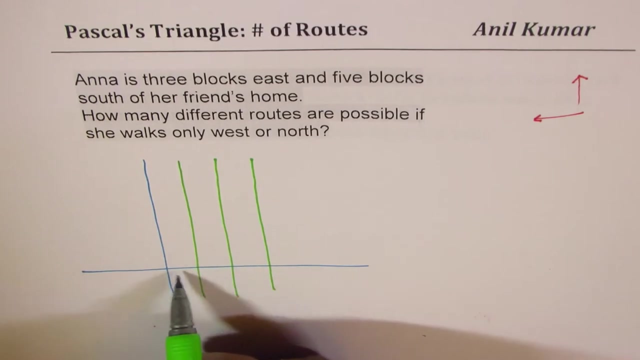 north, Correct, So let's make the grid for us now. so in this particular case, what kind of grid will you have? so let's say, let's make X's first, okay, so Anna stays three blocks east. let me draw three lines here: one, two, three, right, so three blocks is one, two, three blocks? 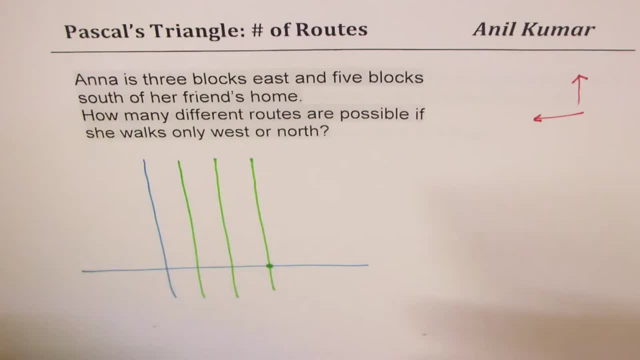 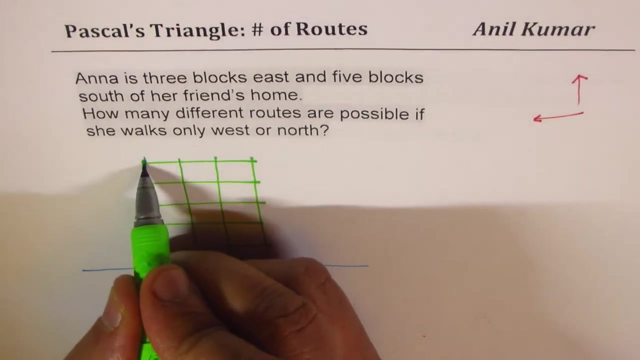 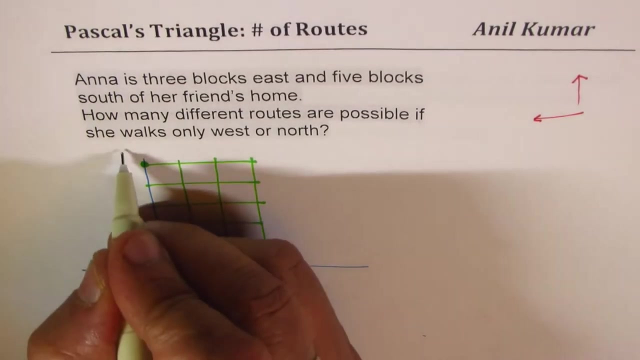 east and five blocks south. that means friends houses in the north right. so we have five blocks: one, two, three, four and one five. so that is the friends house. perfect. so we can mark these two positions, a for Anna and F for friend. and now we'll do find out. 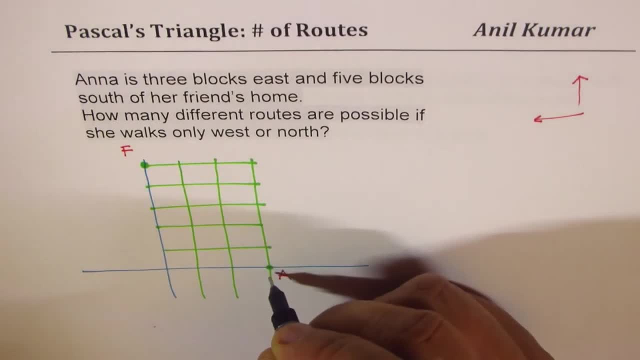 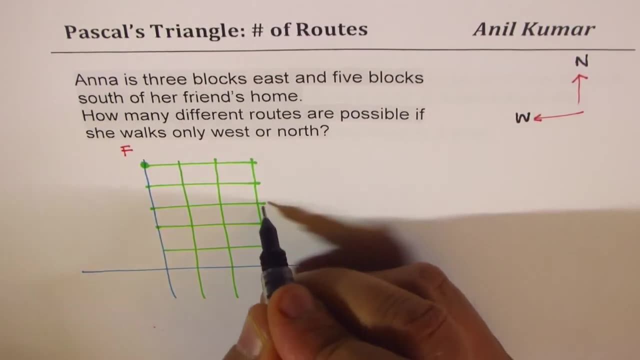 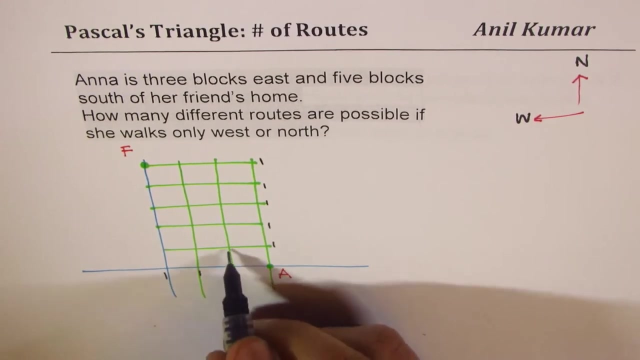 how many parts are there? so if Anna goes straight up north, this is north, and then she can also go west. then be one, one, one, one and one. and as far as West is concerned, from here, one, one and one. now let's go. one one makes it two, two plus. 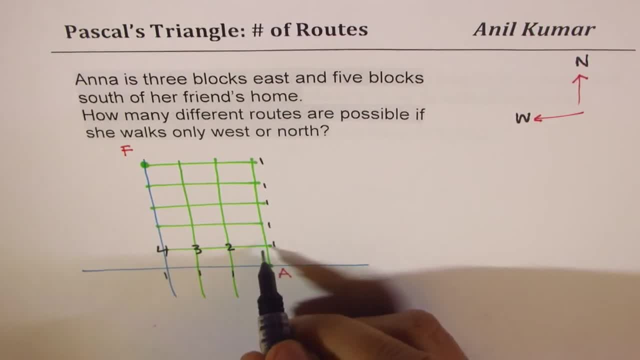 one is three, three plus one is four. now here we could reach this point from these two directions. so two plus one is three, three plus three. so diagonally you have to add correct. so it is three plus three, six. six plus four is ten. come back to the starting point. one plus three is 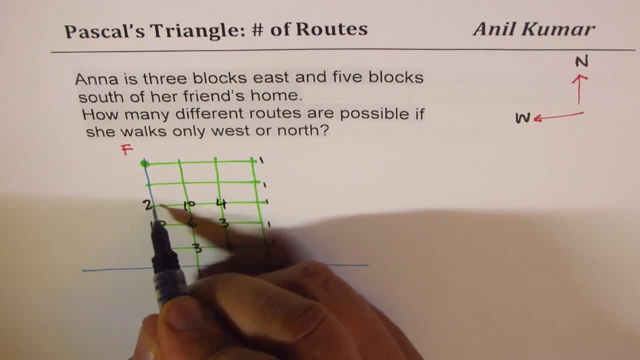 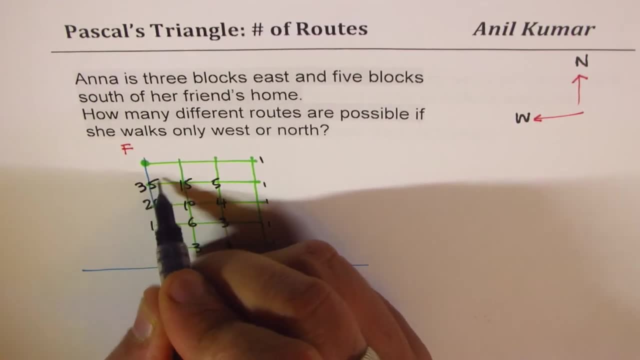 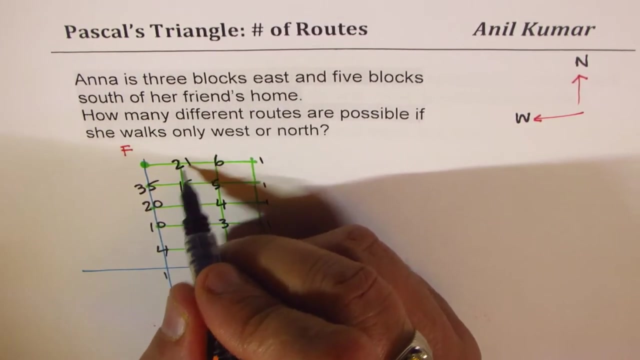 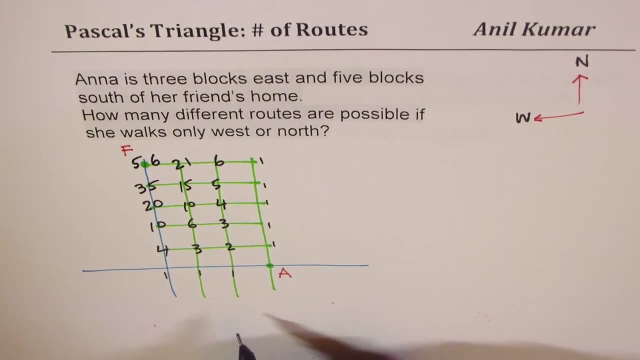 four. four plus six, ten. ten plus ten is twenty. one plus four is five. five plus ten is fifteen. fifteen plus twenty is thirty five. one plus five is six. six plus fifteen is twenty one, and twenty one plus thirty five is six and five fifty six, correct? so there are fifty six ways. so that is how. 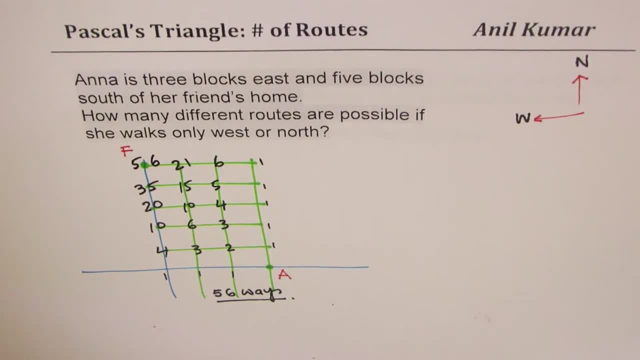 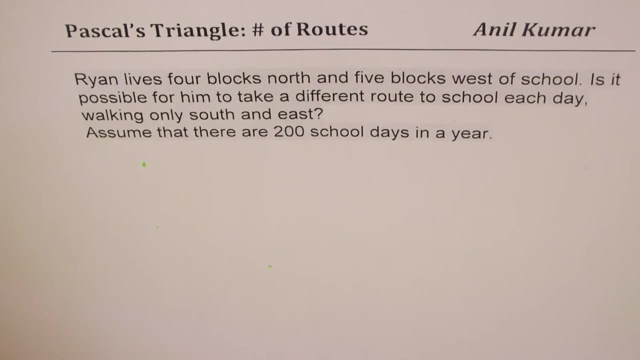 you have to do these questions right. sometimes it may be difficult to you know they may get mixed up, but that's fine. let's see the next question. it is a similar word problem. it says trying lives for blocks north and five blocks west of school, right. so is it possible for him to take a different route to? 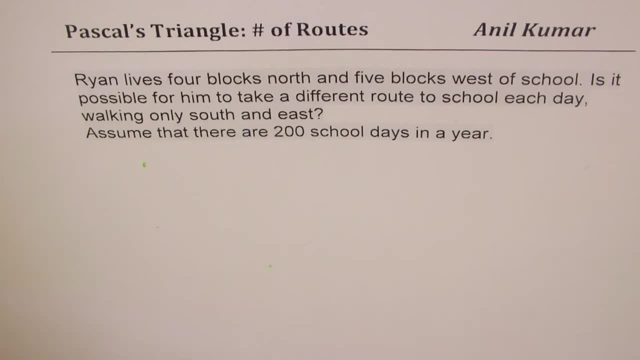 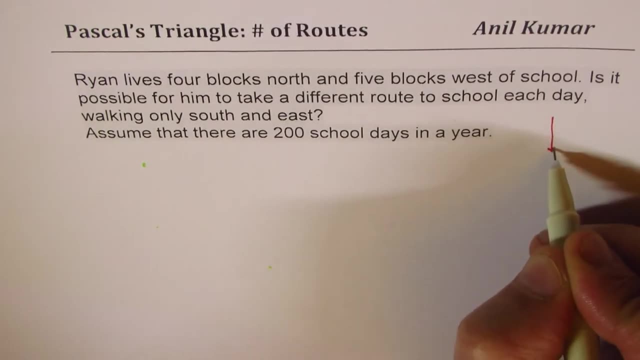 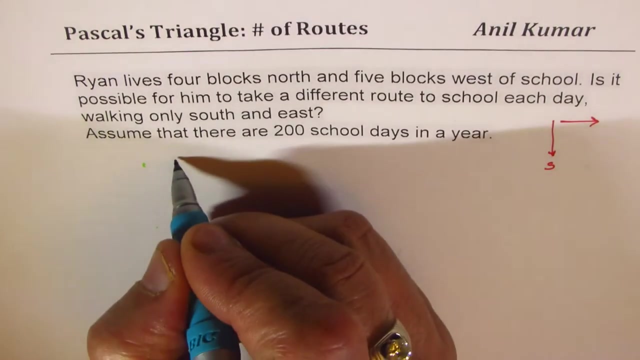 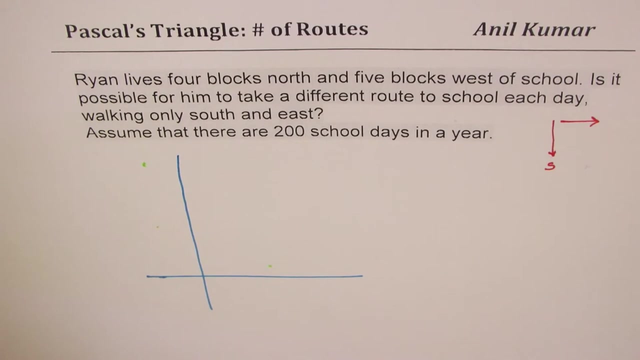 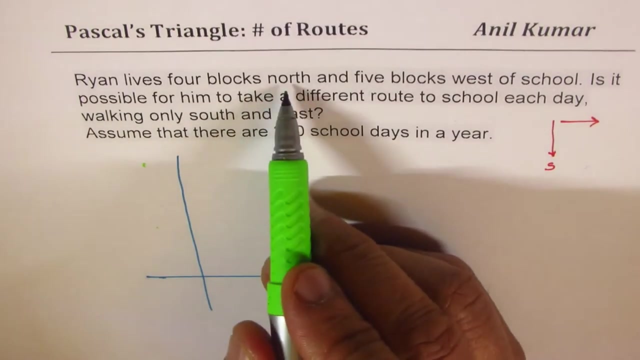 school each day, walking only south and east. assume there are 200 school days, so ryan is walking only south or east, is it okay? and now let's again make the similar kind of a grid as we did last time and then work it out, okay? so ryan lives four blocks north and five blocks west, so school is. 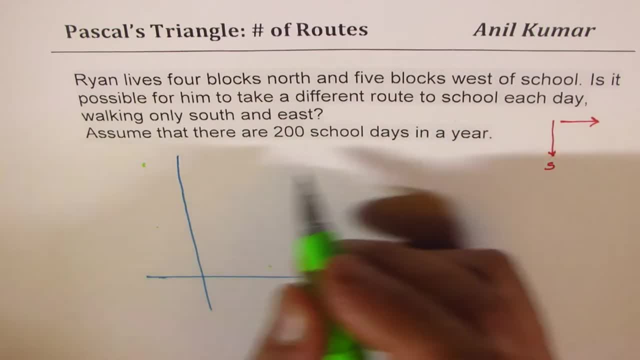 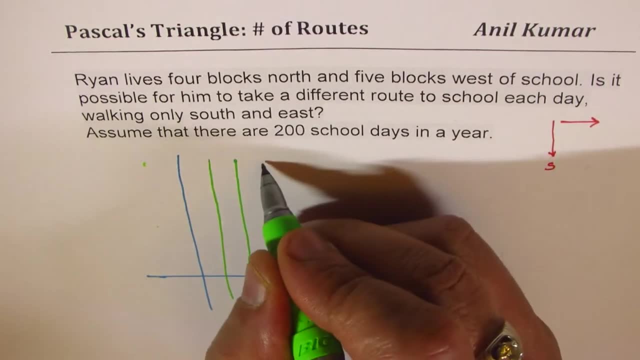 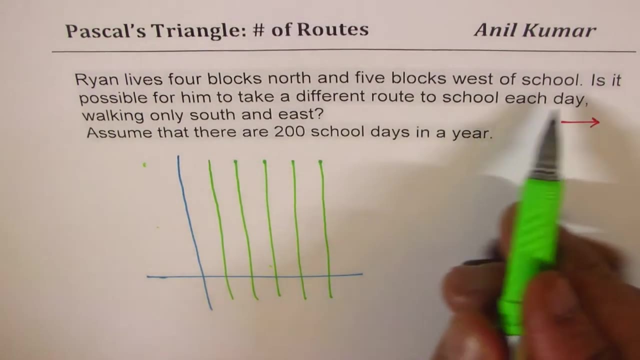 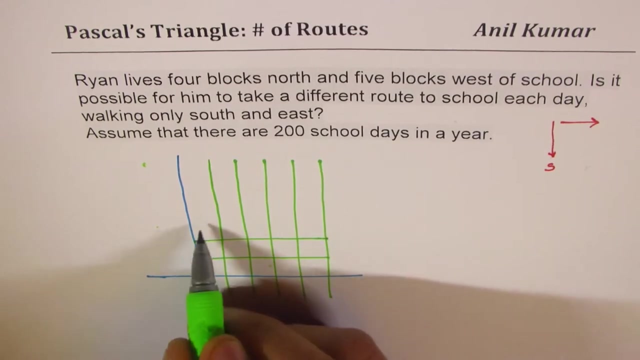 here. ryan is there, so we'll make five blocks first for the school right, so we'll make it towards east: one two, three, one two, three, four and one five. so these are five blocks west, four blocks north. so let's make four blocks this side so we have one two, three and one four right. so we get to the position of ryan. so this is ryan. 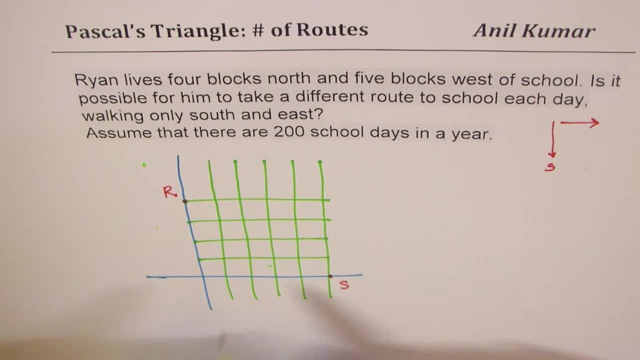 and that is the school. so ryan lives four blocks north and five blocks west. so from here, one, two, three, four north. one, two, three, four, five west is perfect, great, correct? let's write down the numbers. ryan can move either east or south. so if ryan moves south, then it is one, one one. 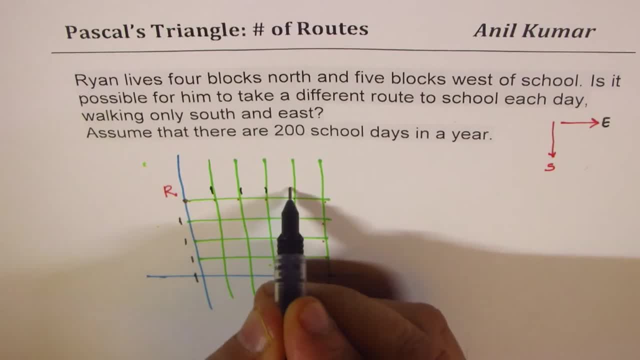 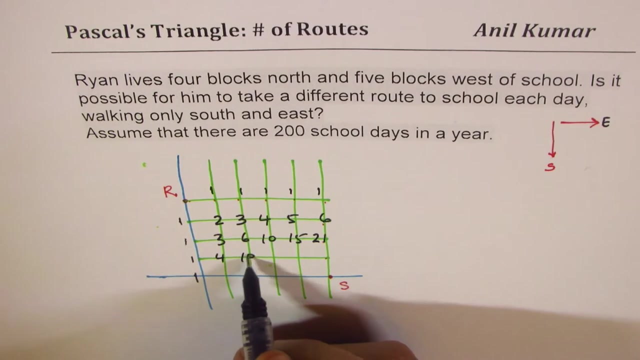 and one. perfect east. it'll be one, one, one, one and one. combined positions: two, two plus one, three, three plus one, four, five, five plus one, six plus 3 is 6, 6 plus 4, 10, 15 and 6 is 21. okay, 1 plus 3 is 4, 4 plus 6, 10, 20, 35. and when you add this, 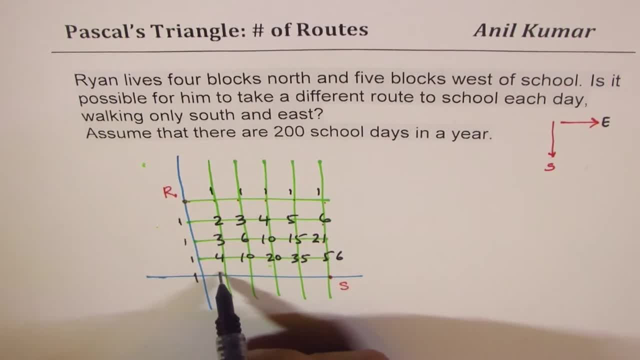 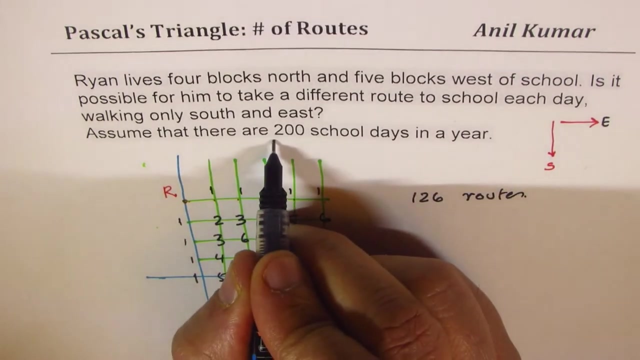 we get 56, 5, 15, 35, 70 and 70, and 56 is, let me write here, 6, 7, 5, 12, 126. so we get 126. as our currency is okay, so there are 126 routes. is it okay? and says: 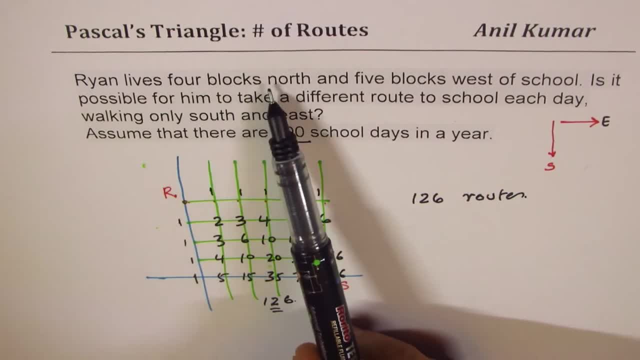 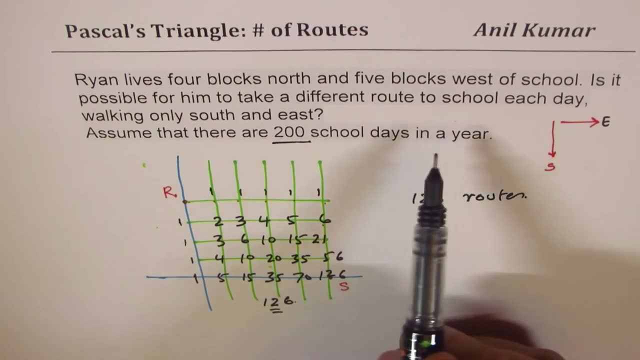 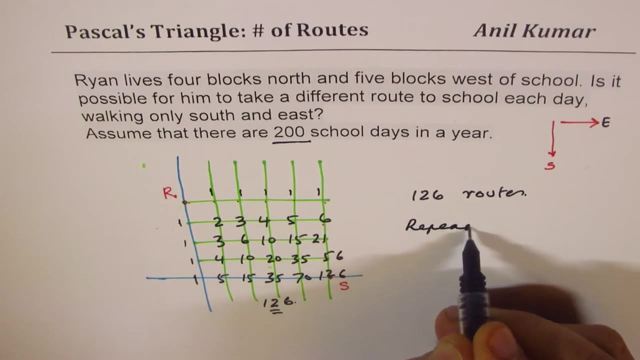 ryan lives four blocks north but he has to go over 200 school days so he has to repeat some. is it okay? so the he cannot go every day with a new route, so so, so he cannot. so he has to repeat. is it okay? so he cannot. 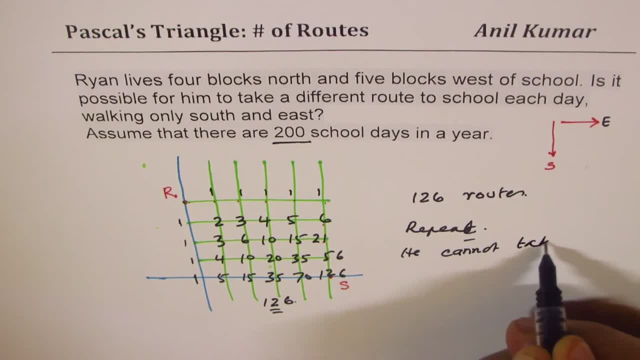 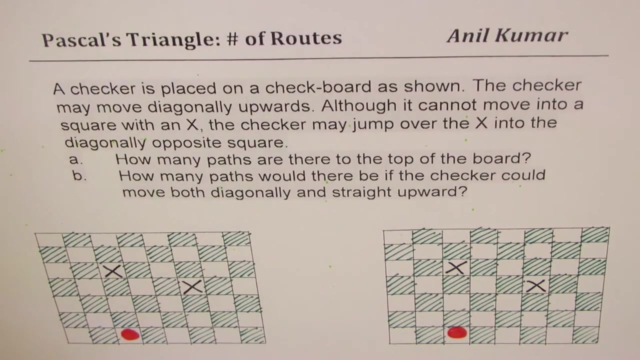 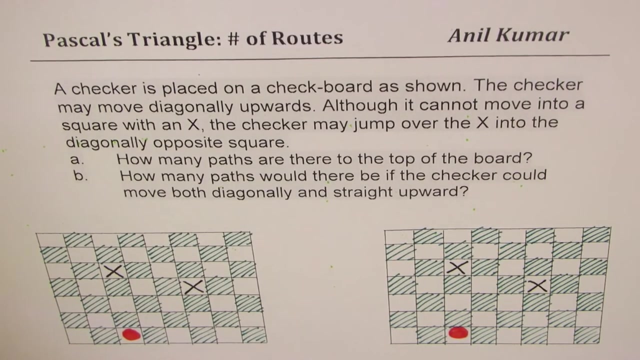 take a new route each day, since the number of combinations is just 126, whereas there are 200 days to go for the school right. so now let's get back to our original. so we are back to our first question, which was the primary objective. we have learned all the methods to do this particular question. a checker is placed on a. 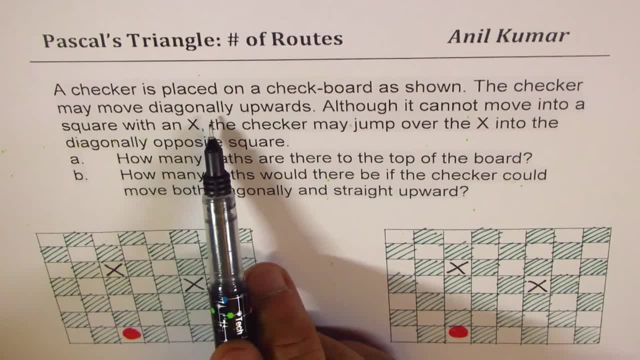 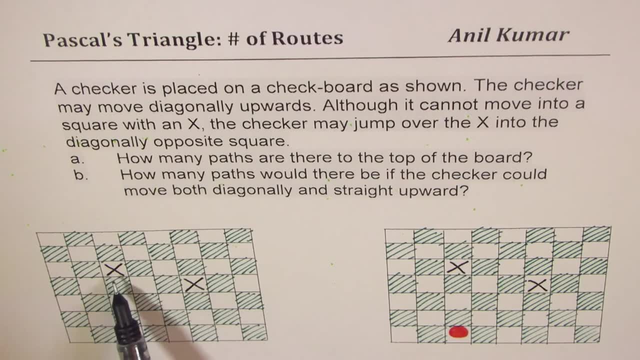 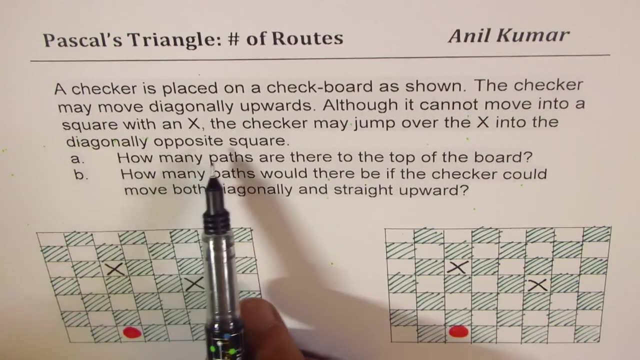 checkbook. as shown, the checker may move diagonally upward, although it cannot move into the square with x. so these are two squares. with x it cannot move into this location. the checker may jump over the x into diagonally opposite square. that means you can go from here to there or from here to this. 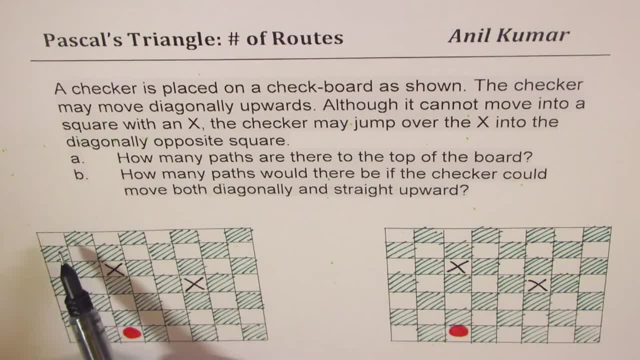 how many parts are there to the top of the board which you have to find? part a, part b is: how many parts would there be if the checker could move both diagonally and straight upwards right? so those are the two parts and accordingly i have two sets of drawings for you. you can actually 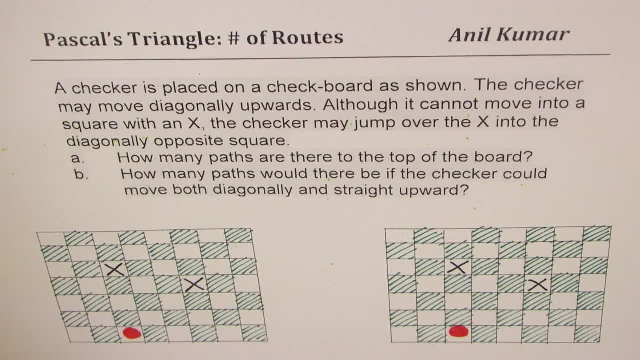 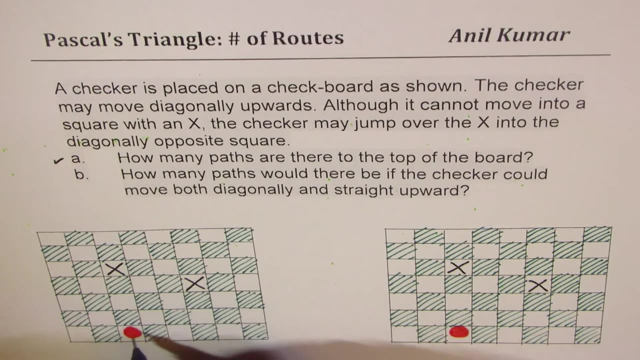 pause the video, figure it out and then look into my suggestions. so i'll keep a calculator handy because we may land up in big numbers here. so let's begin part a checker is there. we can only go diagonally, so best way is let's go diagonally and mark one in all these positions. so it is, let me use. 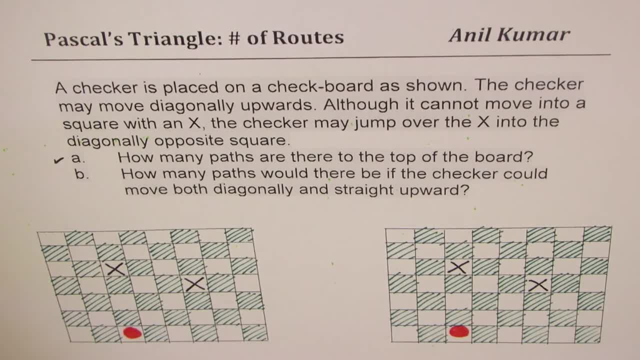 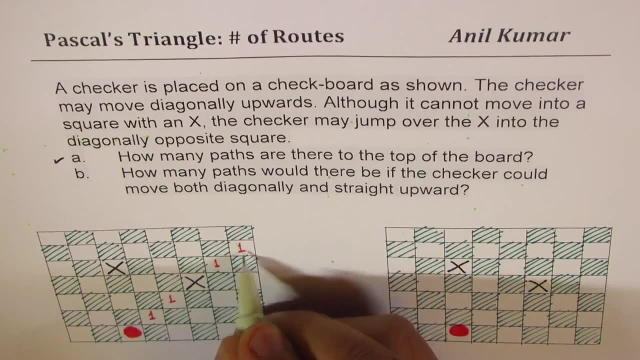 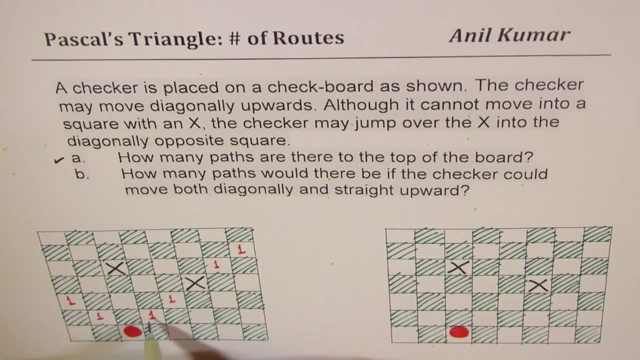 a different ink, okay, uh, okay, let's use red is okay, so we'll mark one. so one, one, one and one right. this side also one and one. now let's look into it. here we can reach from two places, so it becomes two, and then here two plus one. 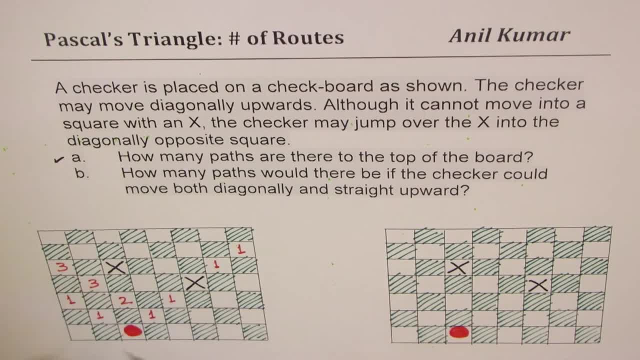 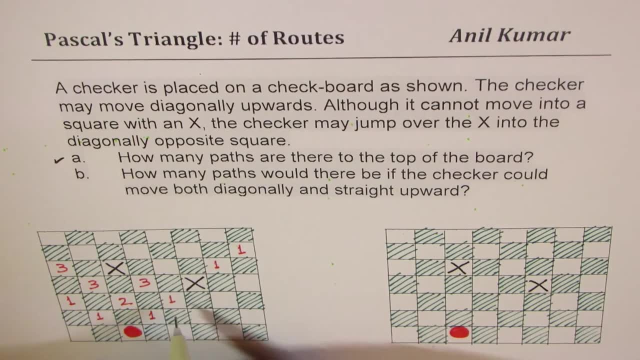 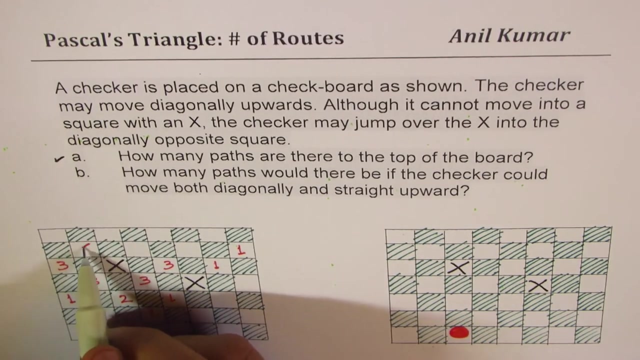 we have three and this place. only three will move in. okay, here, one plus two is three. now this place, we can uh go only from this side. so it is three, perfect. now three can jump. three can jump- come here. three can also come here. so we have three plus three, six in this location. perfect, let's get to. 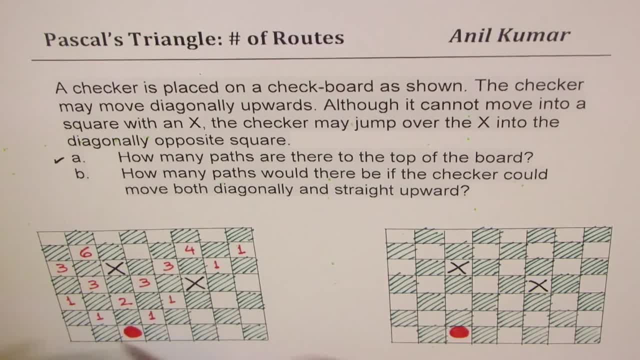 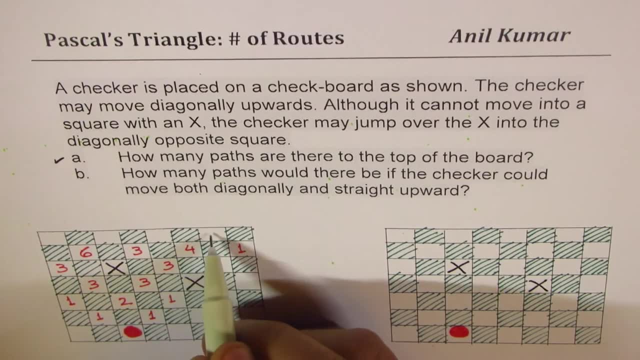 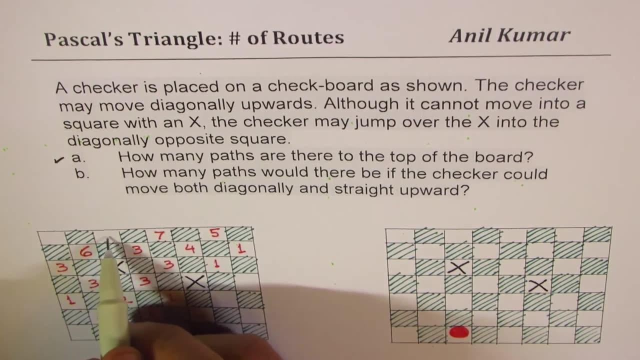 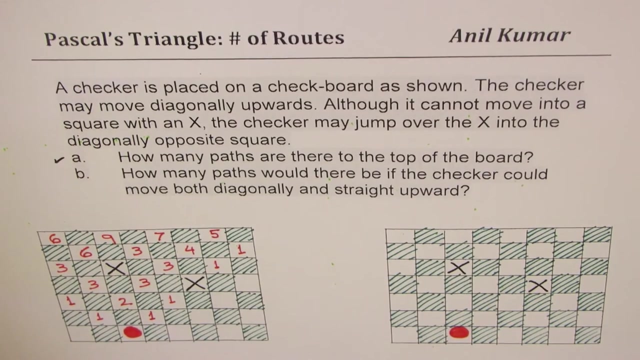 this one plus three is four. here only one way, only three can go there. okay, this place: one plus four, which is five. now here, four plus three, seven, six plus three, nine, and this diagonal: only six can go. so that is what we have and therefore the combination is: we have to add six plus nine, plus. 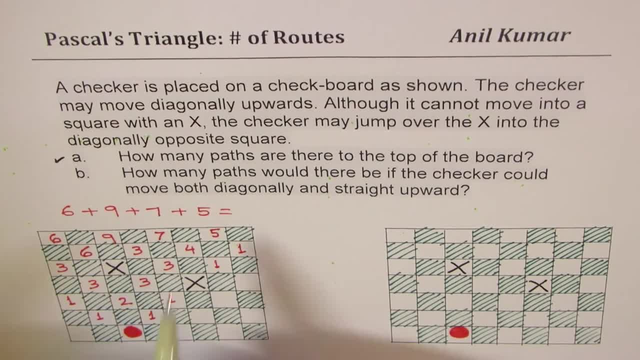 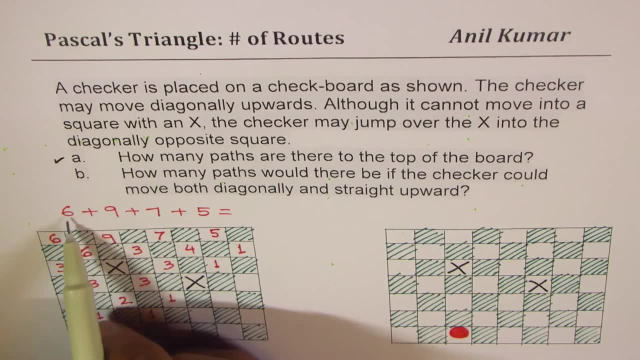 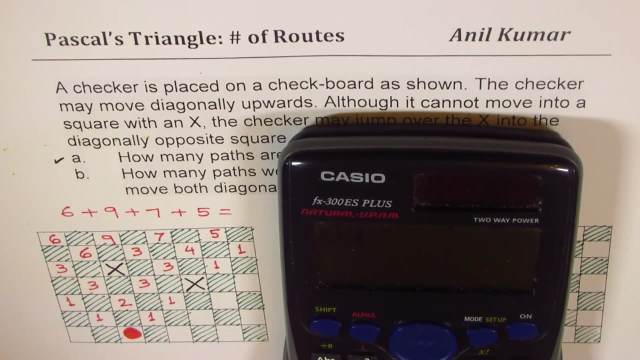 seven plus five to get the result. is it okay? seven plus five is twelve. twelve plus nine is twenty one, and twenty one plus six is twenty seven, correct? so that is our answer. so we'll just add six plus nine plus seven plus five to get our answer, which is twenty seven. 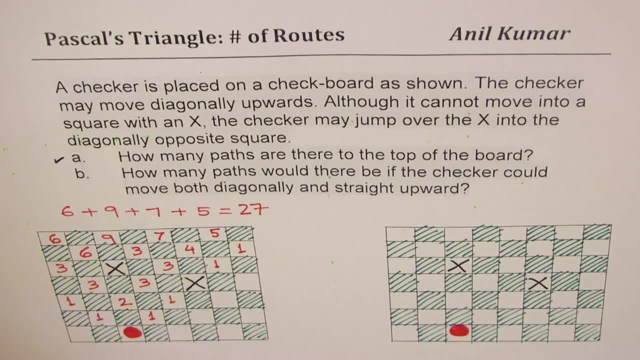 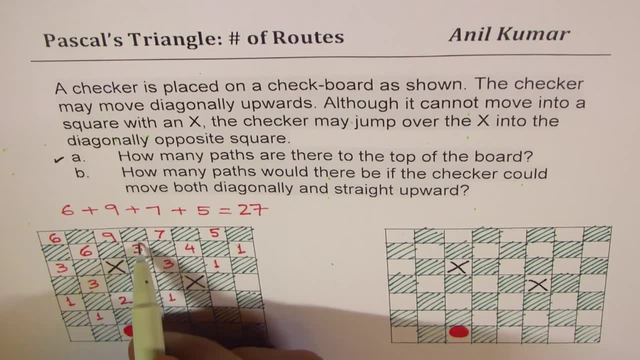 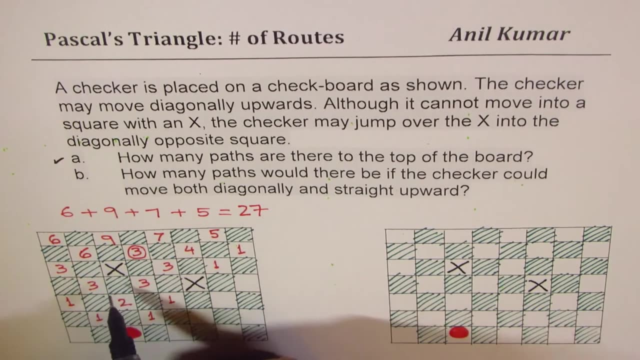 that is how it should be done. perfect. so we're we actually made a mistake here. let me correct this. this position is not correct. okay, so it's good, i saw this, so let us correct this one. so here you could actually also reach from this place. so it is three plus three, so this should. 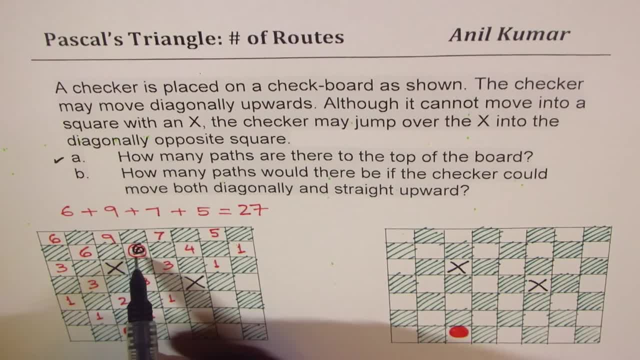 have been six, so let me make six here. and when this becomes six, then some other numbers will also change. six plus four, this becomes ten for us, and here we'll have six and six as twelve. so this becomes twelve for us. so those are the corrections, since you can jump right. so i forgot to add this three. 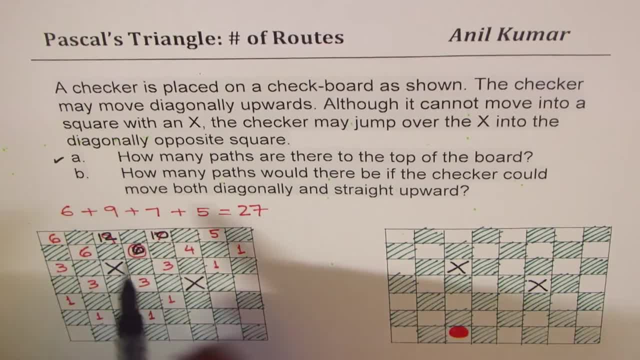 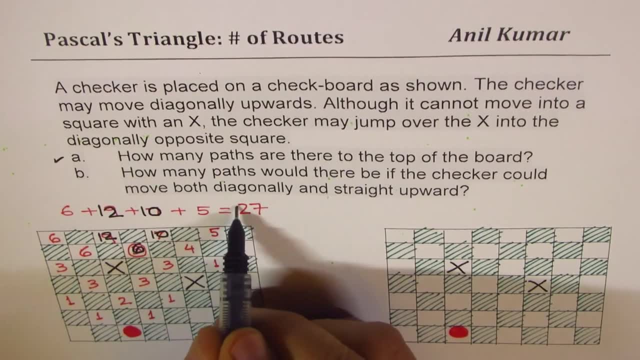 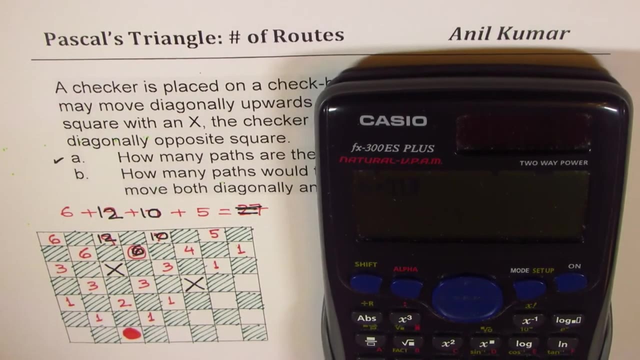 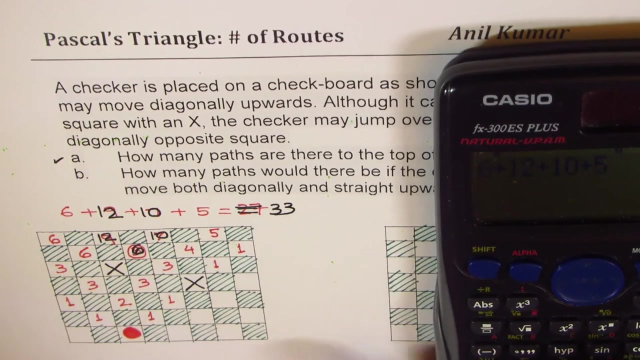 in this particular location and therefore these numbers are now six plus twelve plus this is not seven but ten, and the number will change. so let me correct it. so we have six plus twelve plus ten plus five, and the result is thirty three. so we get thirty three as our answer and not twenty seven. okay, so i hope you understand. 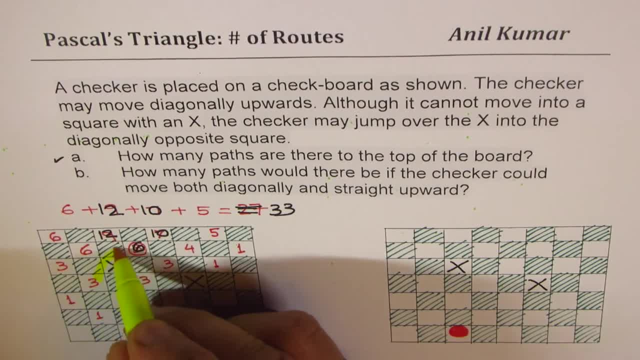 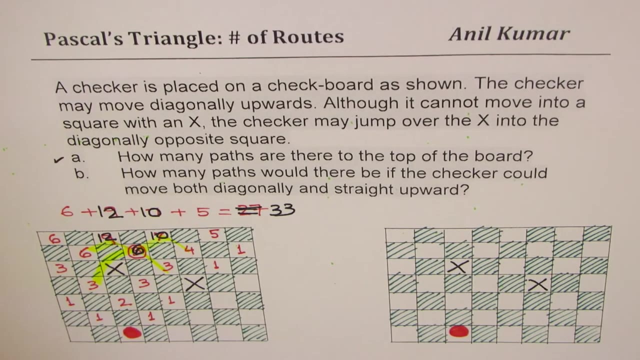 what was the mistake? we could jump over this, so this three could go from here and this could also go. both will give us six. once we get six here, then six and six is twelve and six and four is ten. perfect, so be careful when you do. you may or may not get exactly same answer. if you don't get recheck, okay now here. 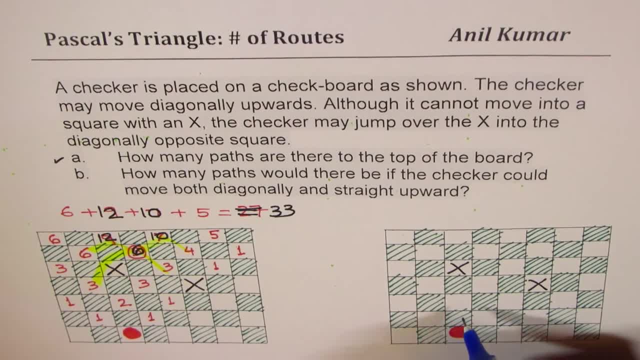 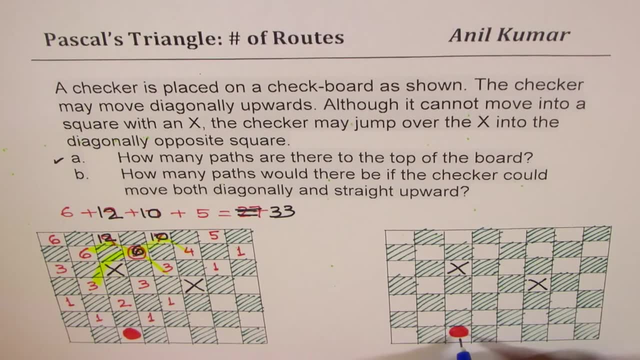 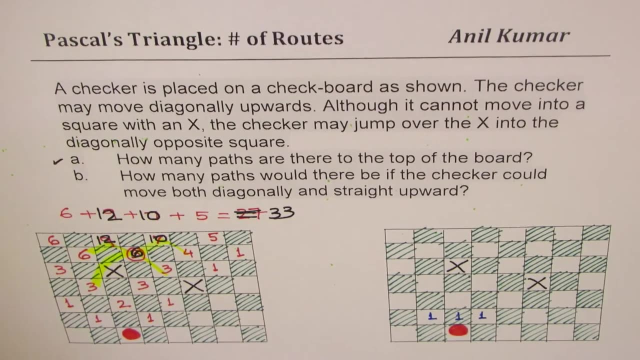 let's get into the second one here. so this time we can actually go up as well as diagonally. so let's go from here. going up means one, do you see that? diagonal also one, and left also one. so we'll go a bit slow here. now for this position. 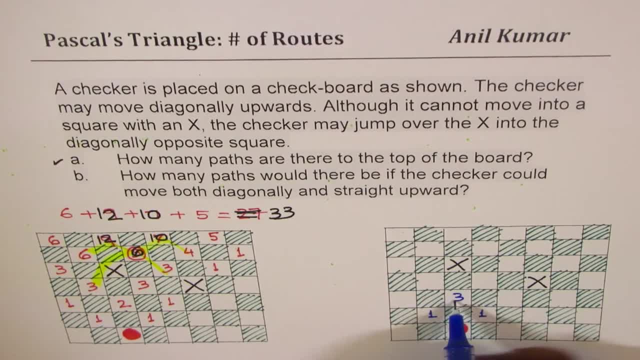 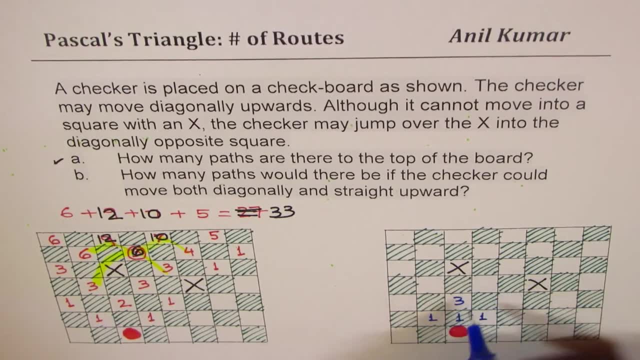 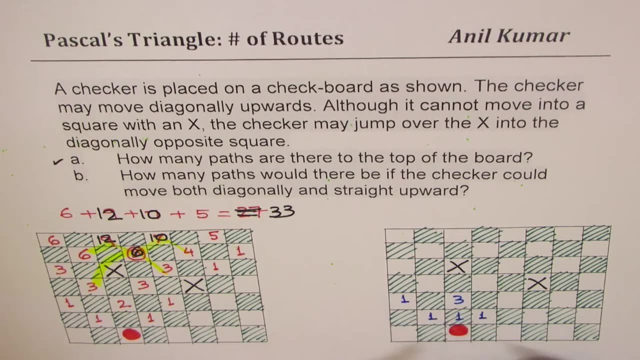 we can go up and diagonal also, so we have three ways of getting to this position. correct now, three ways getting to this position. if i here, we get only one way, so one is perfectly fine. now, in this position, we could come from one and from here, so that we get one plus one is two. 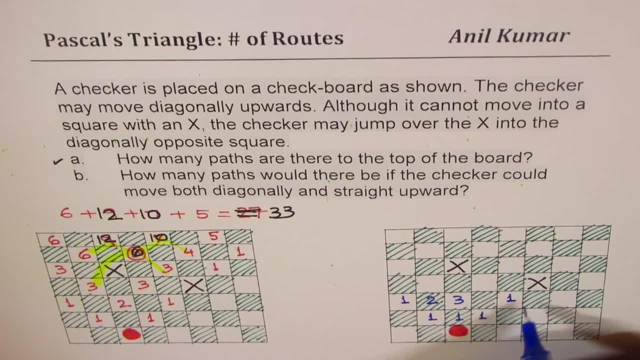 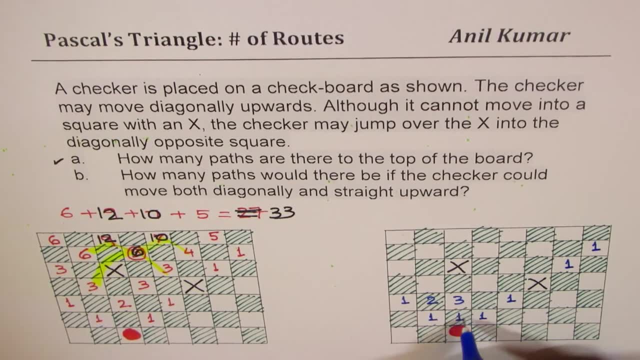 now, moving right is not a problem, only one, jumping it is one, and then going one. that is safe. now, here we could go from two places now up and diagonal, so we have two, now again up or diagonal, so we have two plus one. three. here we could come from three positions. so three plus three is six. 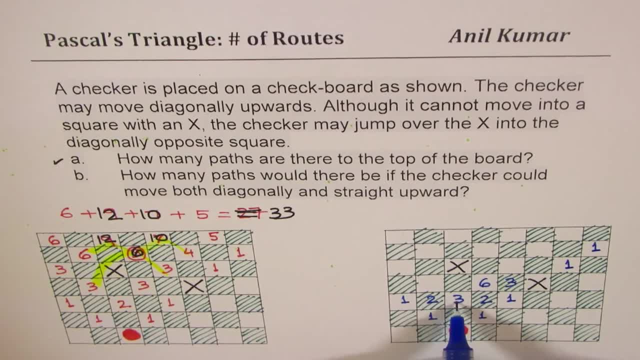 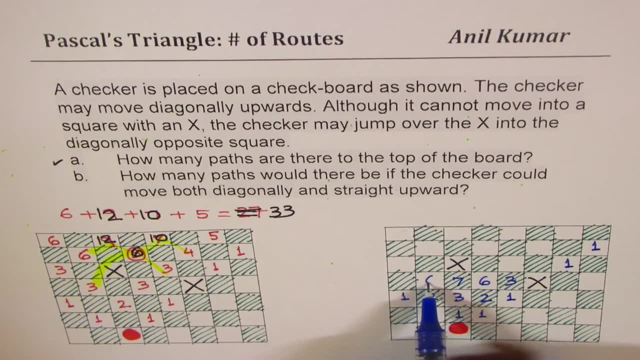 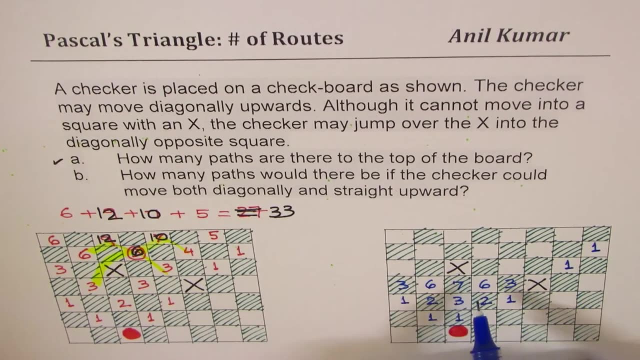 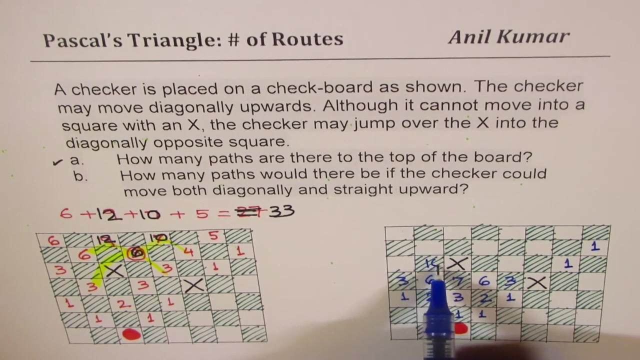 now this position can be occupied by two, three and two, which is seven. now, here it could be combination of three, two and one, which is six, and here it could be two and one, which is three. okay, next level, uh, next level. so here we could go from these three, so just 16 corner, six and three, nine. 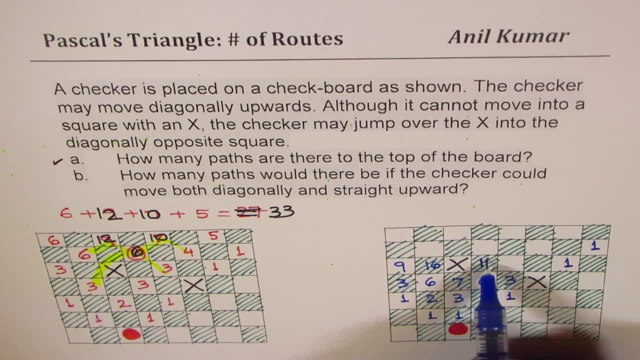 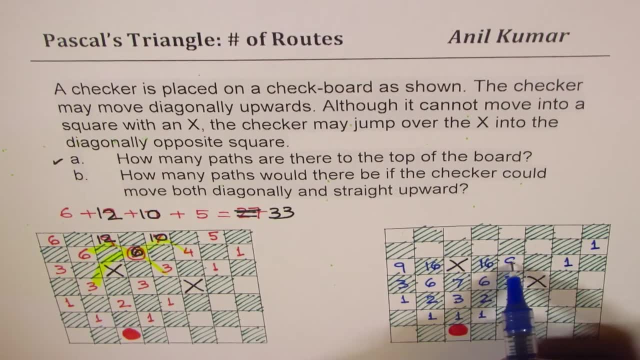 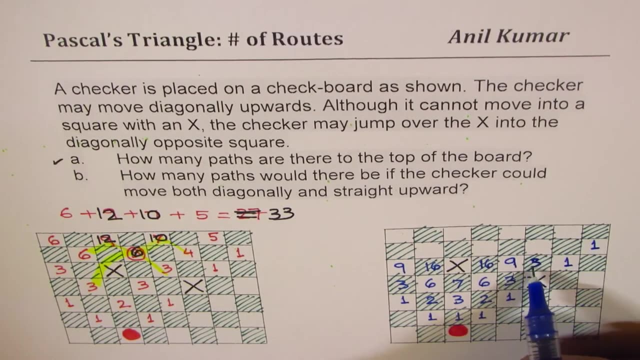 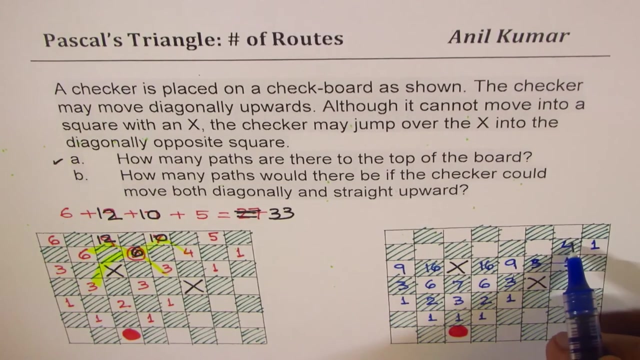 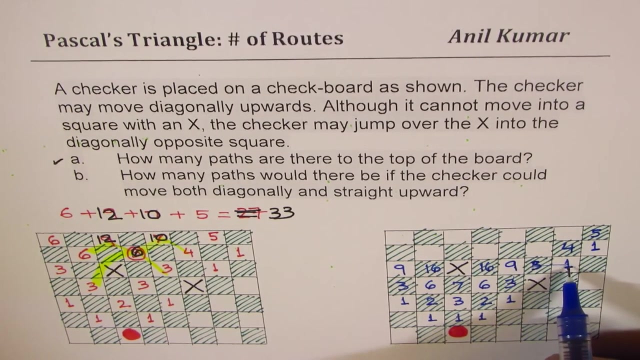 here: seven, ten, sixteen. this position three and six, nine. nothing is here now. this position is only for three. okay, now coming to that position: three plus one, four. this position, four plus one, five. here it is diagonal three and so thirteen. here we have to add these three: 19 plus 9, 28. 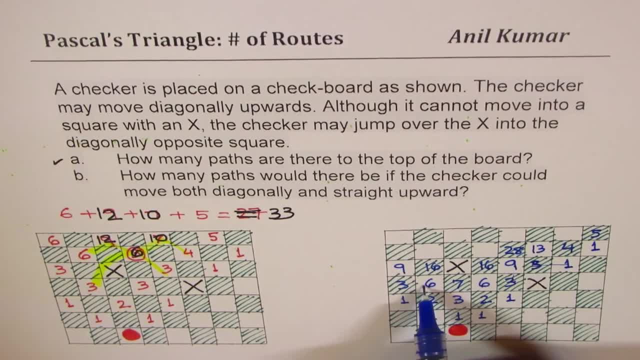 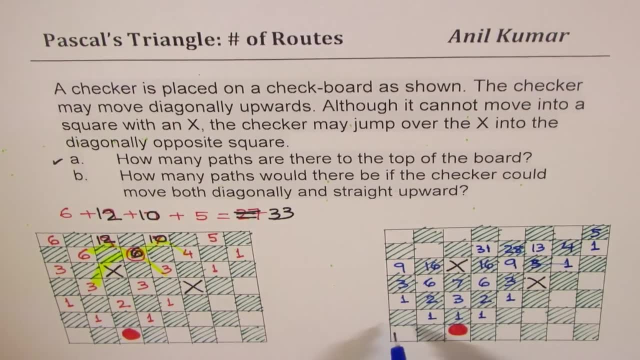 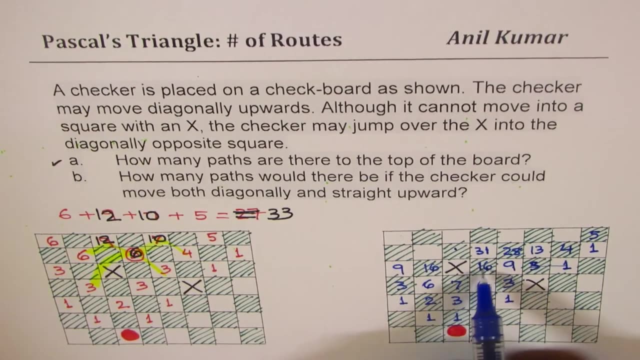 this position we have 9, 16 and 6 because you can jump and come right. so 6 and 16, 22 plus 9, 31. now next position: 7 could jump and come: 16, 16, 32 plus 7, 39. 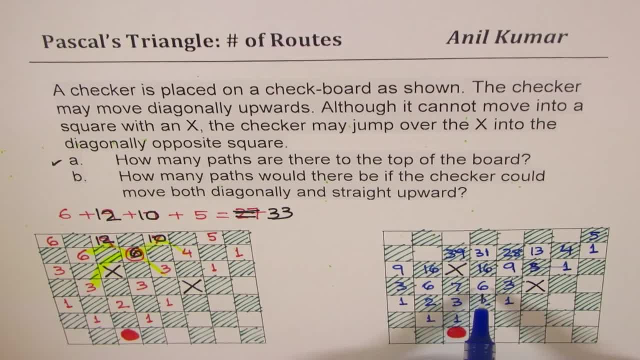 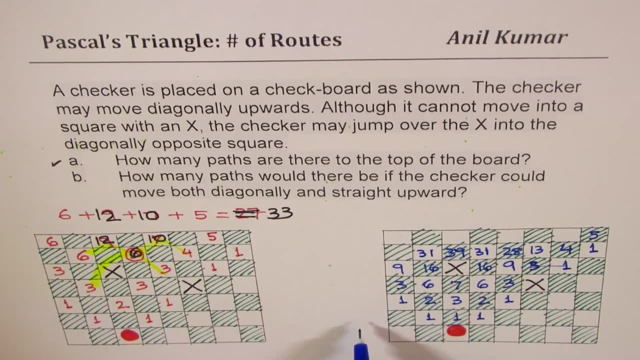 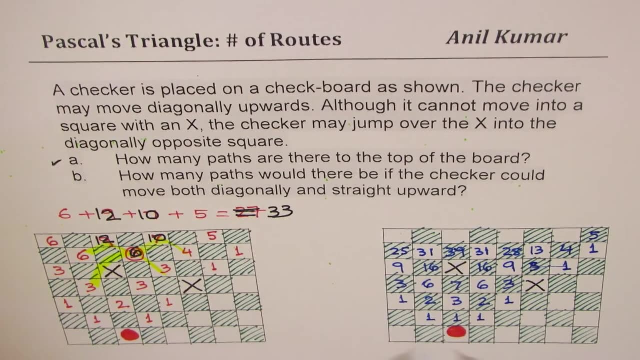 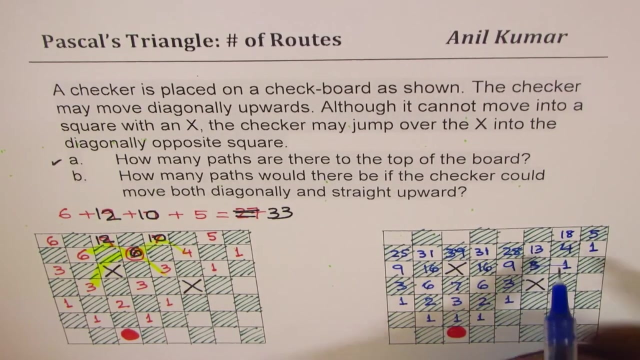 okay, 6 can jump and come. so we got 6 plus 16, 22 plus 9, 31, corner 16 and 9, 25. okay, so we are close. three positions: 5, 13, 18, three positions again, so let's add, so 28 plus 4, 32. 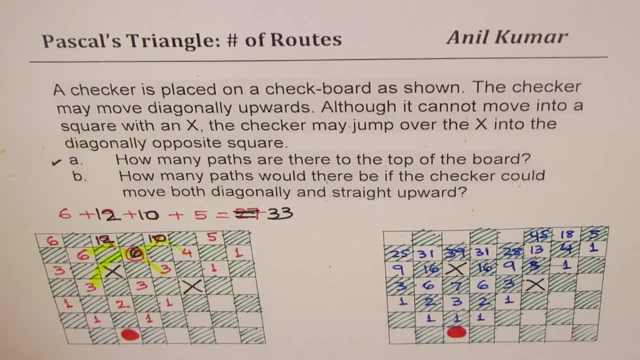 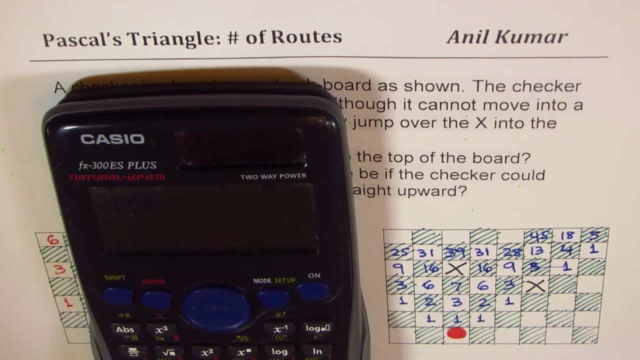 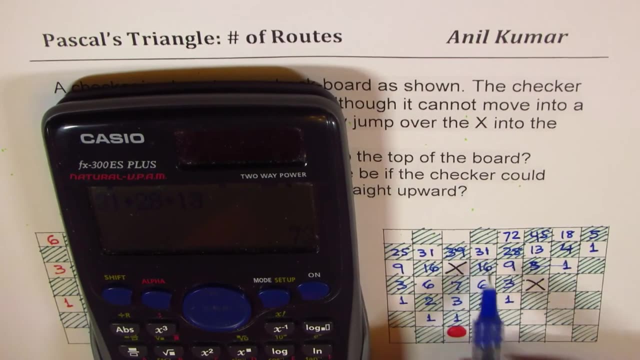 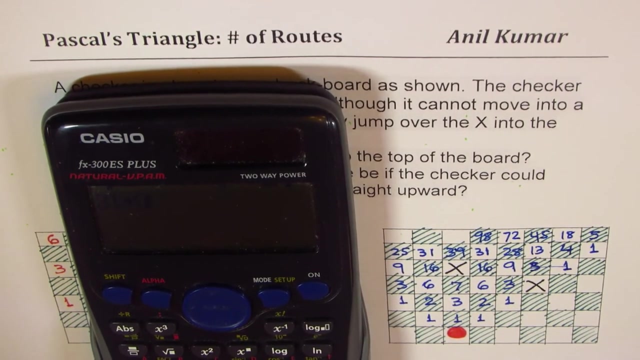 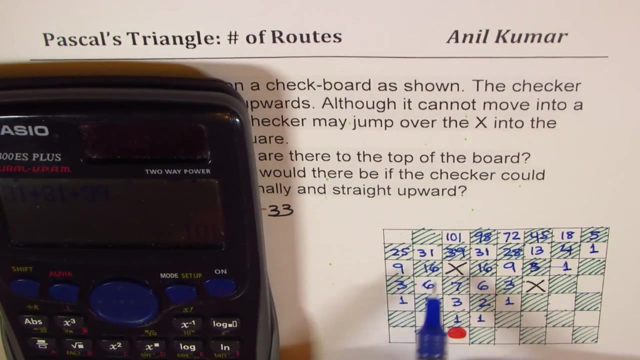 45. here let's add with calculator: okay, so 31. let me add 31 plus 28 plus 13. that gives us 72. here here, 39, 28, 31, 39 plus 28, 31, 98. next position: 31, 31, 39, 31 plus 31 plus 39, 101. so lots of numbers here: 39, 31 and 25, 39 plus 31 plus. 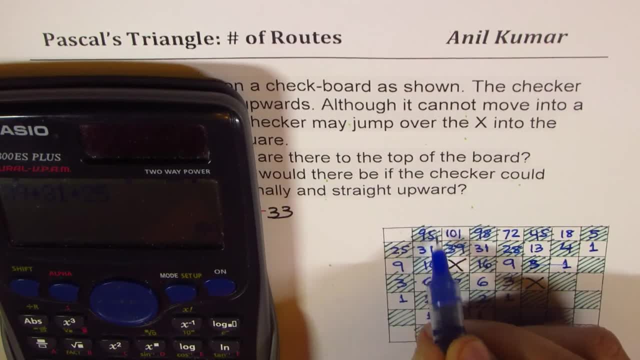 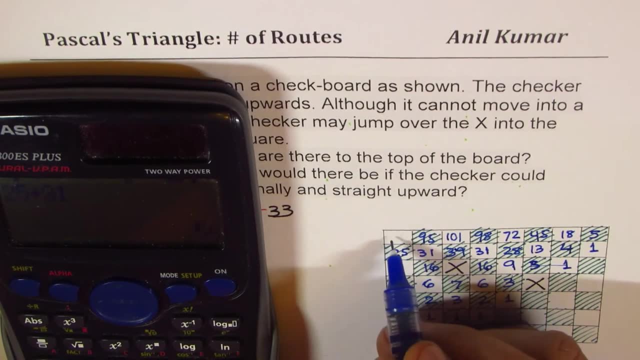 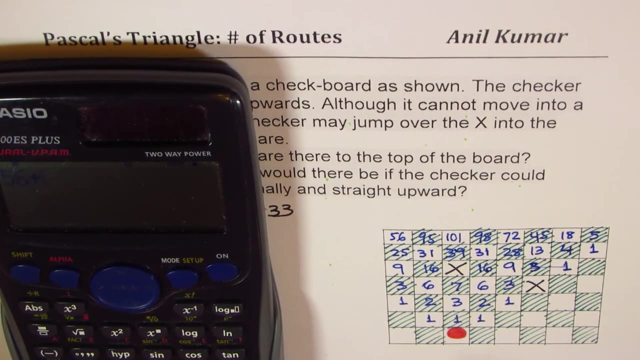 25, 95, the last portion here- 25 and 31, 56. let's add them all, we get 56 plus 95 plus 101 plus 98 plus 72 plus 45 plus 18 plus 5 490. okay, so with my interpretation of, 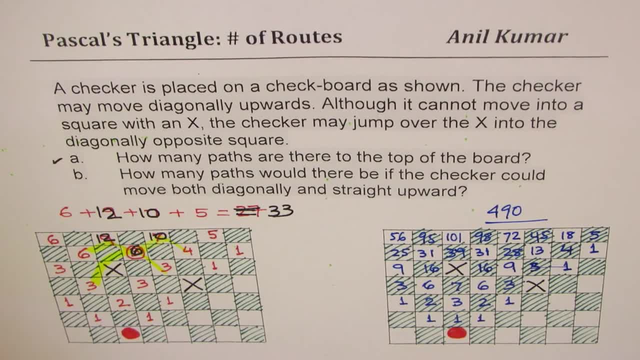 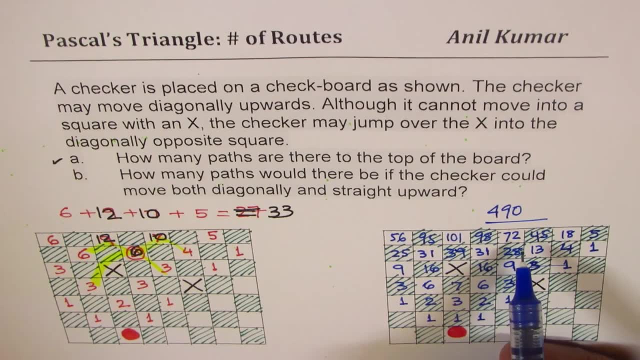 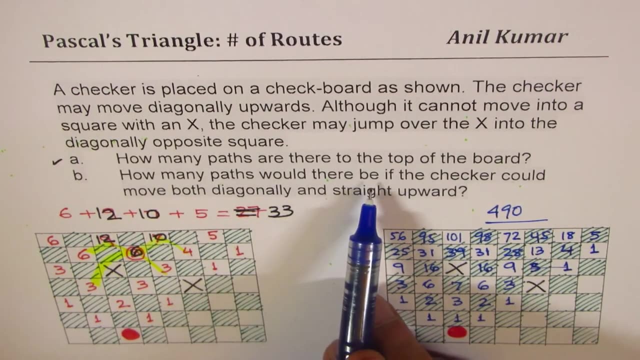 the question. right, 490 is the answer, but I hope you understand the method. I might have done some calculation mistakes, that's okay, but it seems to be correct to me. so what I get here is 490.. So when you say, how many paths would there be if checker could move both diagonally?